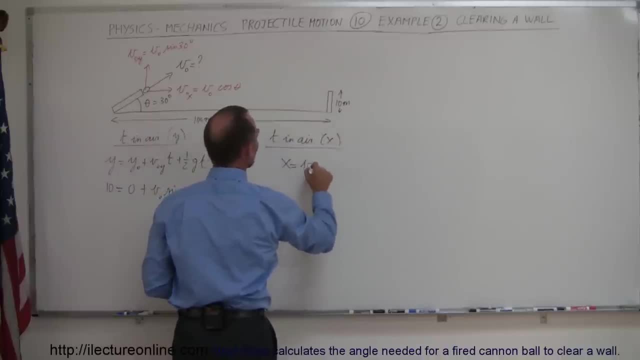 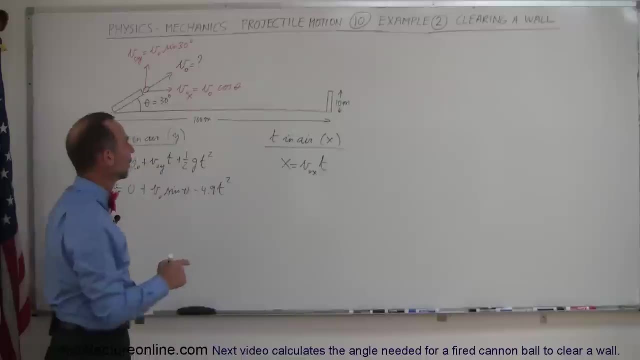 x direction. it would look something like: x is equal to v, initial in the x direction times the time, and of course time appears there as well. So let's go ahead and plug in what we know here. We know that x is going to be 100 meters and v initial in the x direction. that's going to be v. 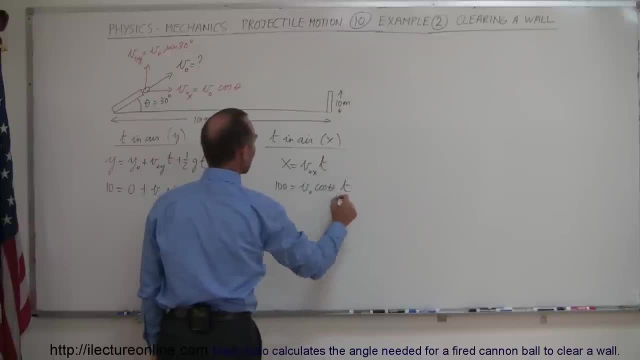 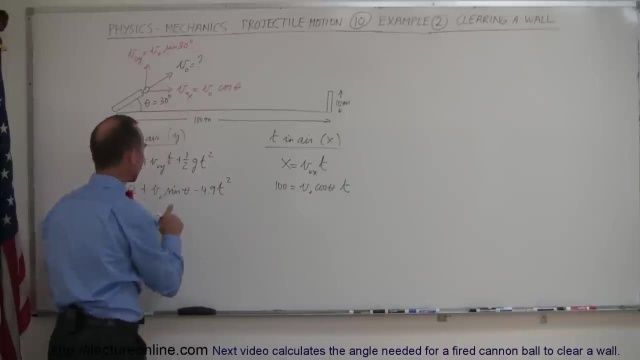 initial times, the cosine of theta times the time t. If we now solve this equation for time and plug it into our equation right here- and oh, notice that I forgot my t here, I can't do that, got to have a t in there as well- If I then plug it into here and here, then I can eliminate. 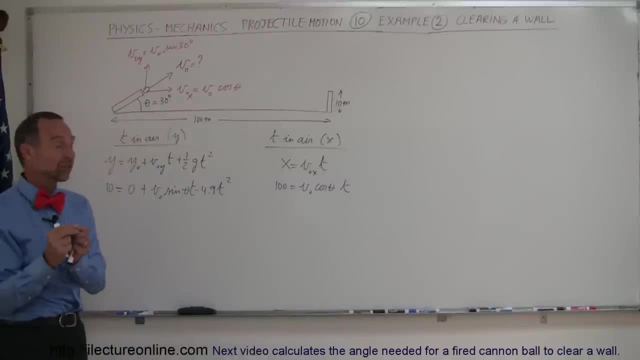 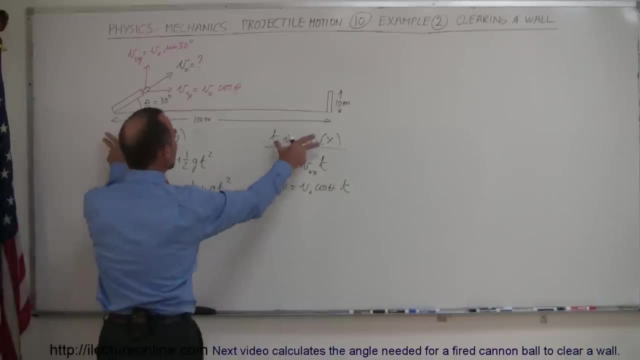 time, and then I only have an equation with v initial as its only variable and I can simply solve for v initial So kind of in a roundabout way, by using time in the air for both the y and the x direction. I can actually eliminate the t and I can then go ahead and solve for the only. 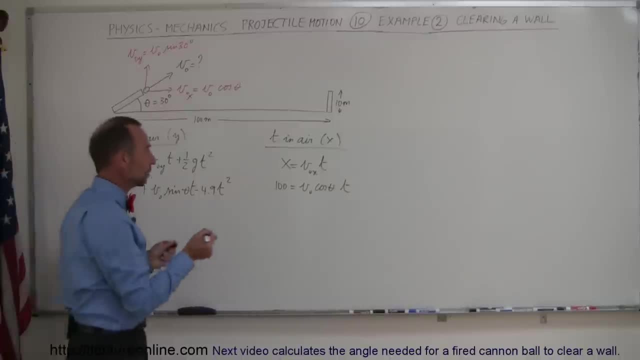 variable- I don't know that's left- which is v initial. So here we can say that t is equal to 100 divided by v initial times, the cosine of theta, and we'll plug that back in here. So that gives us n is equal to v initial times, the sine of theta, and instead of t I'm going to write this right. 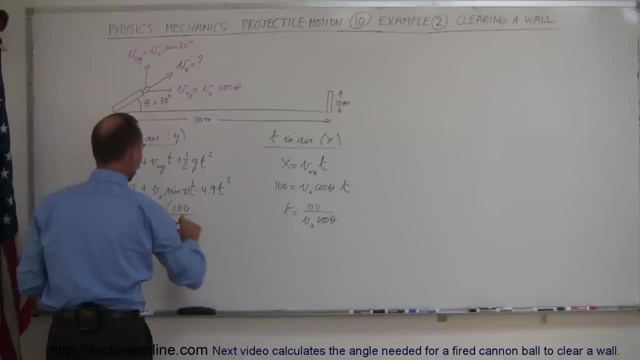 here. so times 100 divided by v initial times the cosine of theta, and then minus 4.9 times t squared, which is this quantity: 100 divided by v initial times the cosine of theta, and the whole thing squared. So now I have to simplify this. Notice that v initial and v initial cancel out. 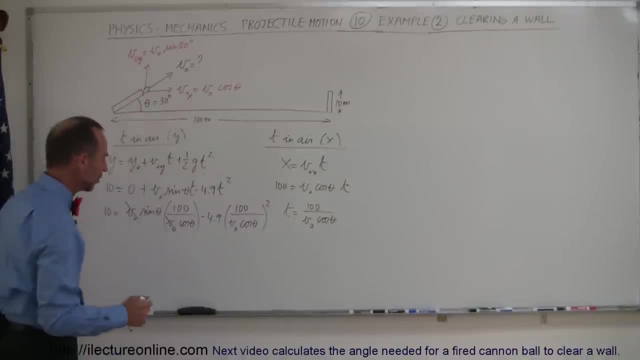 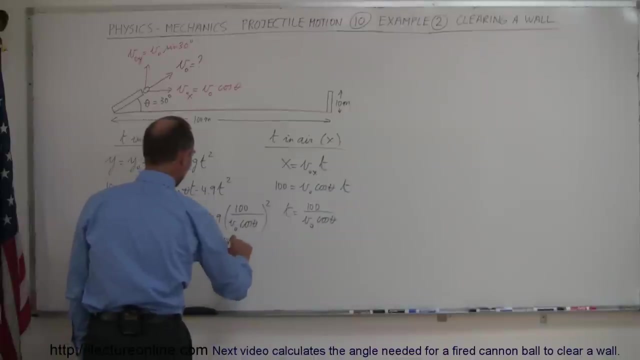 The sine and the cosine. well, the sine divided by cosine is the tangent of theta. so this becomes: 10 is equal to 100 times the tangent of theta, which is of course 30 degrees, in this case, minus 4.9 times 100 divided by v initial. 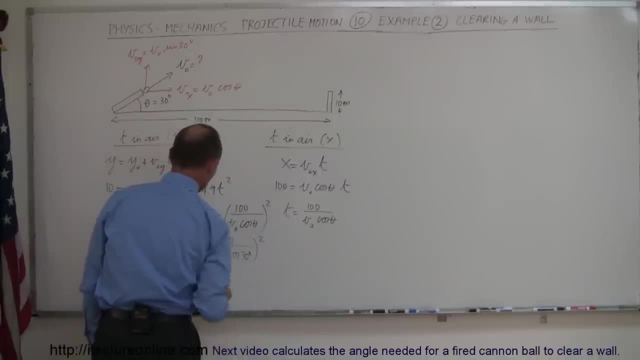 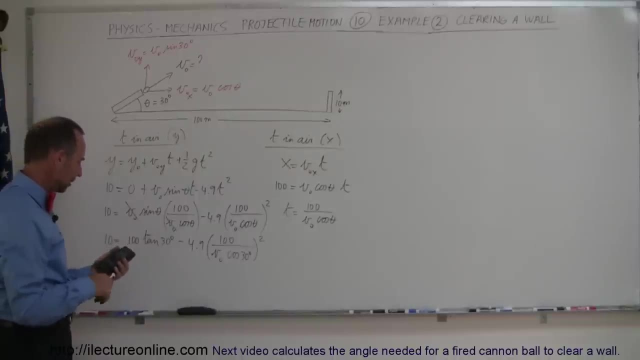 times the cosine of 30 degrees and square that, So I have 30, take the tangent of that, which is 0.577 times 100.. All right, so now I have 10 is equal to 57.7 minus. now I'm going to multiply all this out and divide it by v. 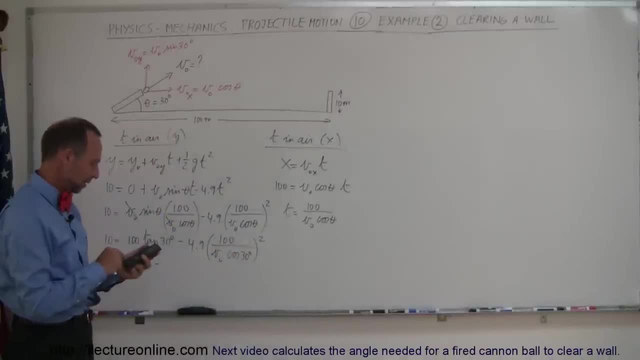 squared, because of course v is squared here as well. So 100 divided by the cosine of 30, we square, that we multiply times 4.9.. Okay, so this is equal to 65,333 divided by v, sub-naught squared. All right, now that looks a little bit better. 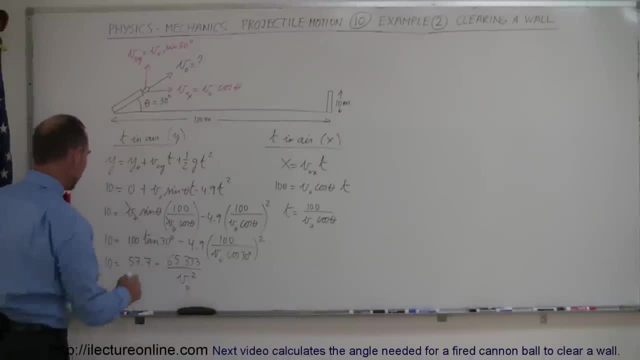 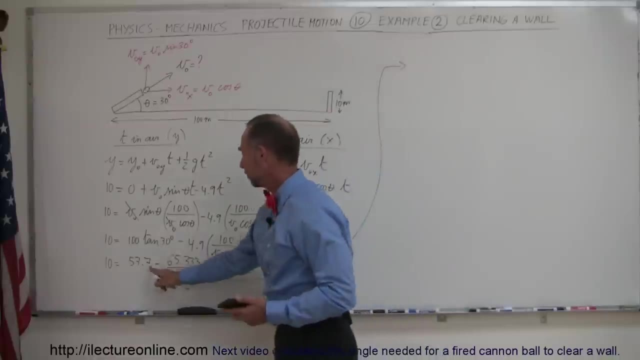 because now I'm simplifying this- I have v sub-naught that I'm solving for, So let's move this across to the other side. So now- and I need some room, so I'm going to move it over here- move the 57.7 over becomes minus 57.7 plus 10, which is minus 47.7,. 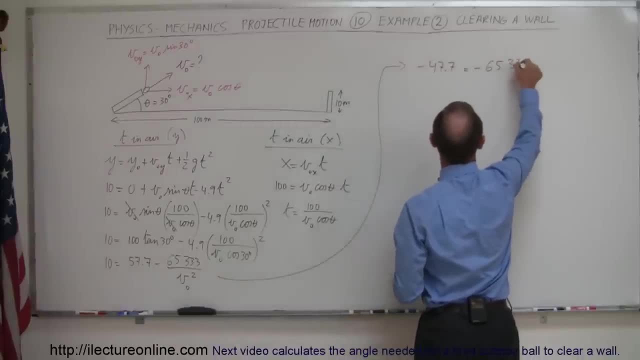 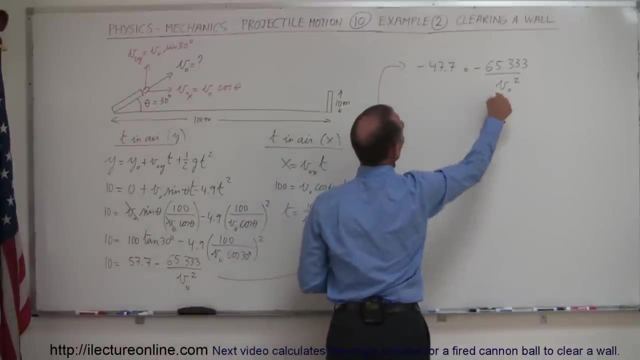 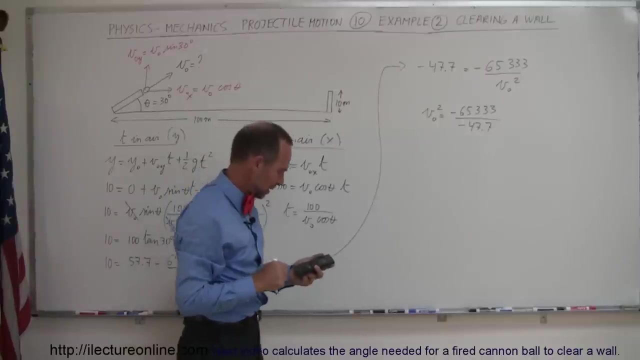 equals minus 65,333 divided by v sub naught squared. the next step is to move this over here and this down there, so we have: v sub naught squared is equal to minus 65,333 divided by minus 47.7,. notice here that the negatives will cancel out, so divide this by 47.7, and then 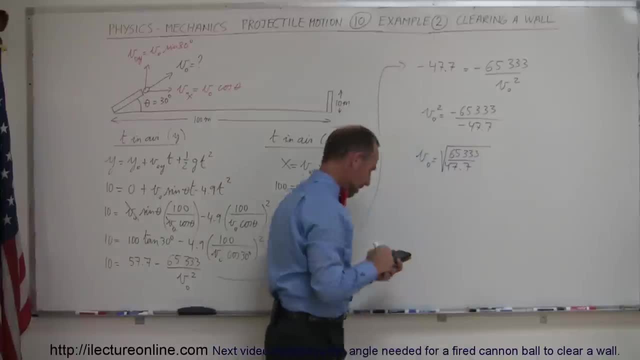 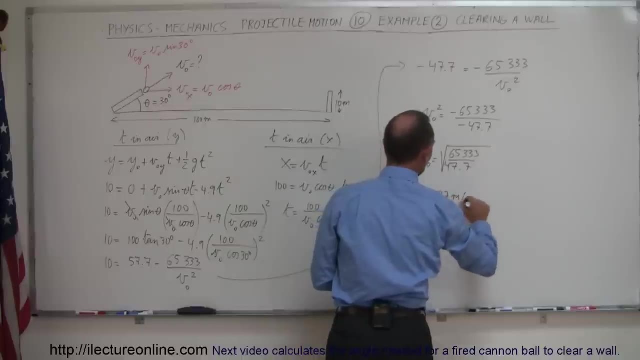 of course v sub naught is equal to the square root of that, and then take the square root and I get 37, so v sub naught equals 37 meters per second. okay, notice that of course I left off the units to make all this a lot cleaner. this would look really ugly when. 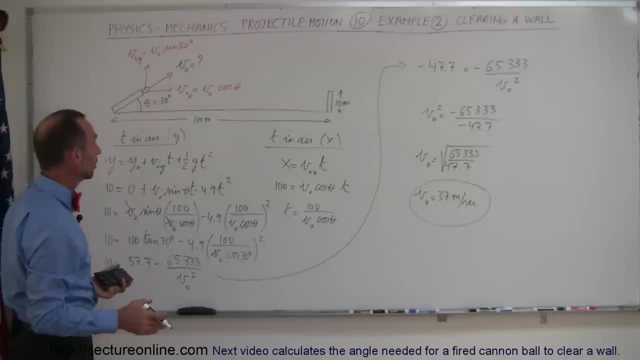 you keep the units in there, but eventually the answer is here. so, even though we started out by solving for time in the air and we realized that we couldn't do that because time was not known and v initial was not known- if we did that then we would get 37 meters per second and then we would get 37 meters. 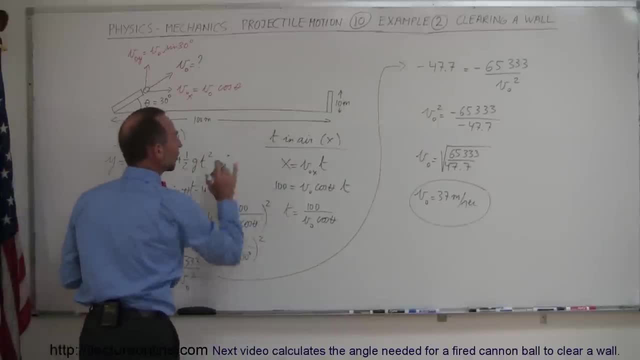 per second, and then we would get 37 meters per second, and then we would get 37 meters per second. so if you then solve it simultaneously by doing the y and the x direction at the same time, solve the equation in the x direction for time. plug that into the t and t squared. 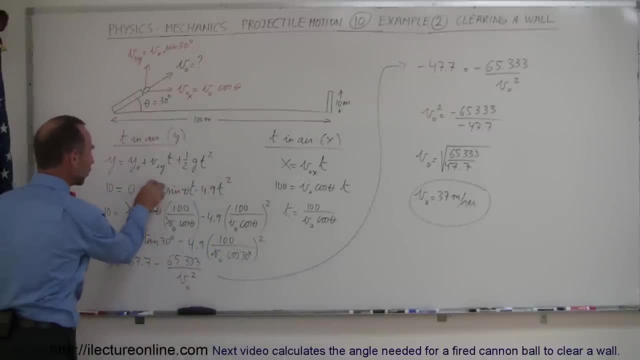 here for the equation for the y direction, and then you are left with only one unknown v sub naught. solve for v sub naught and get the answer. and that's how you do a problem like that where you are trying to clear a certain height at a distance with a projectile.